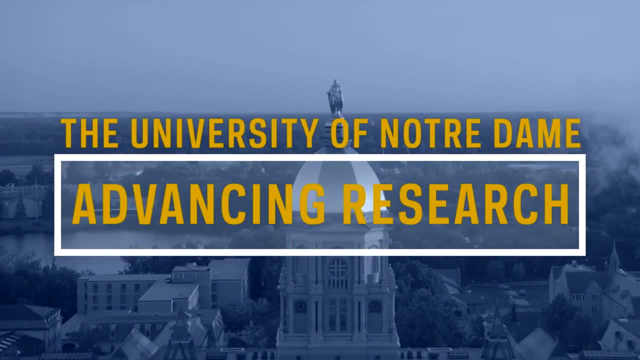 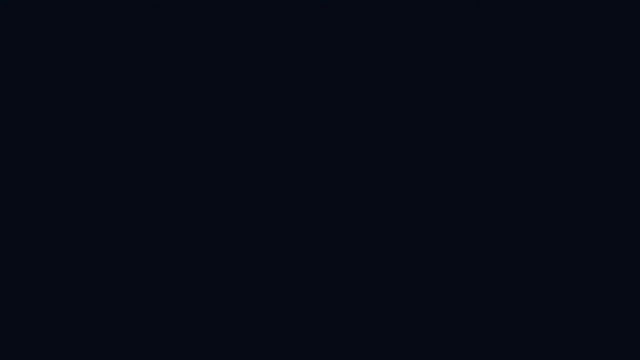 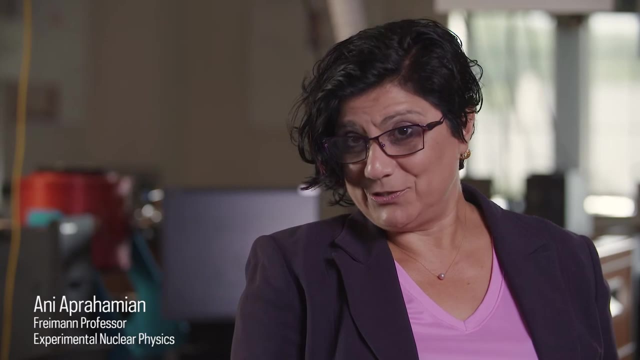 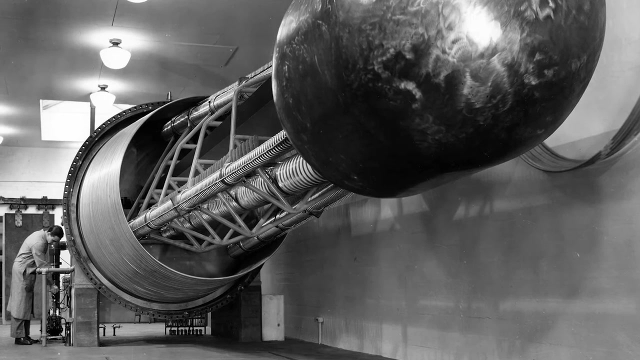 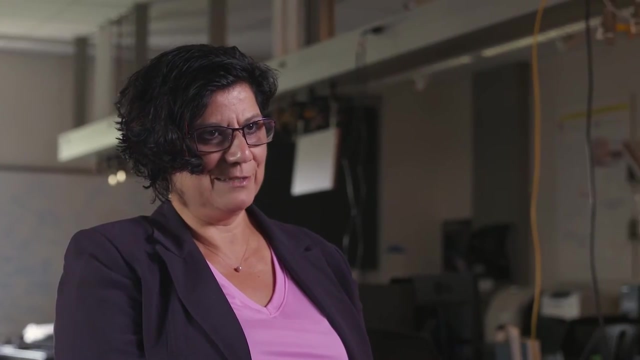 Nuclear physics at Notre Dame has a long history. From the very beginning of the field, actually from the mid-thirties. there was an accelerator here. We decided together to form a bigger vision of where we were going and concentrate on both hiring people and also running experiments. 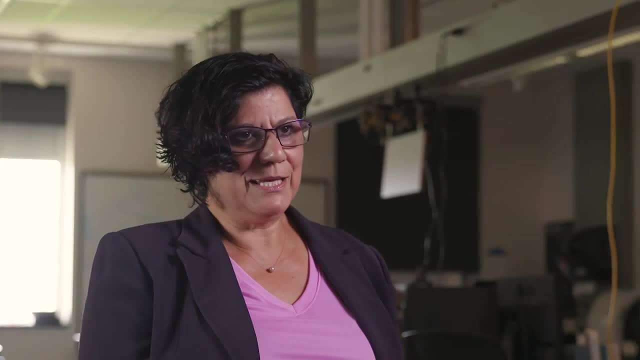 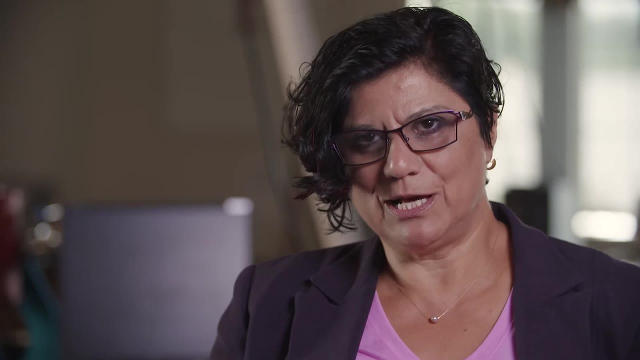 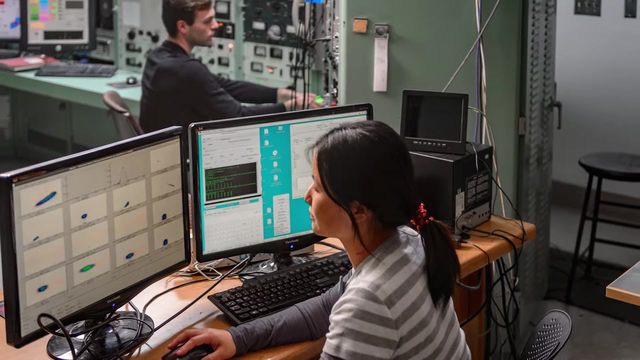 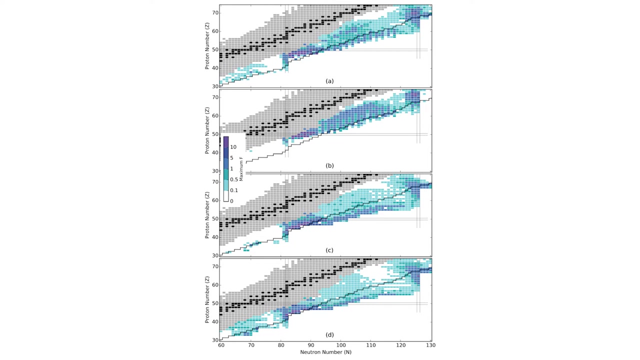 in our facilities. Nuclear physics at Notre Dame has many aspects. We look at the entire sort of birth of stars, the evolution how stars live and die, to how they contribute to the evolution of the cosmos itself. It's a really central focus for nuclear physics all over the world. It's not just us at Notre. 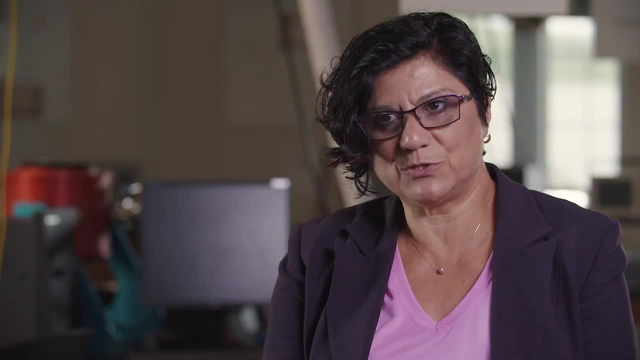 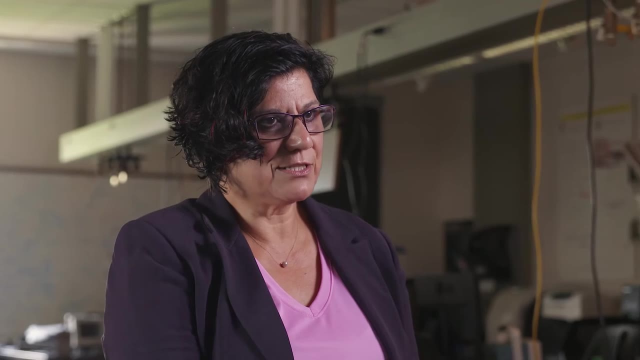 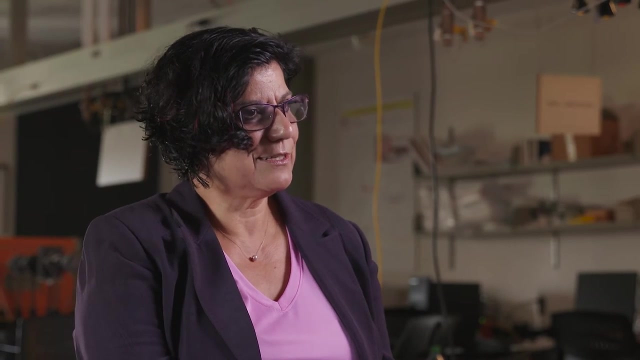 Dame that are interested in it. The facility that's being built at Michigan State- the FRIB had a major motivation of it- was to try and study very neutron-rich nuclei that are potentially produced in the air process. It's no longer that an individual area of 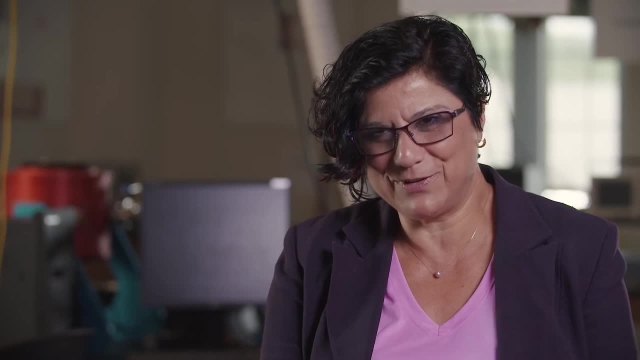 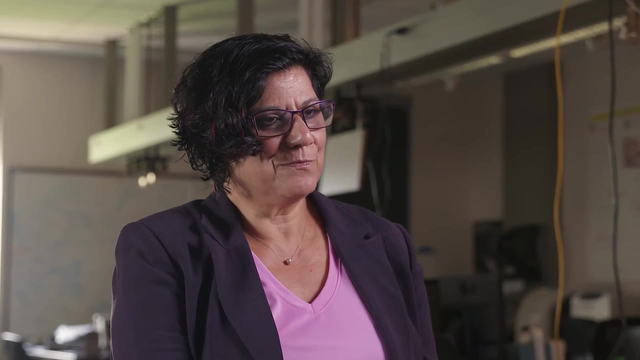 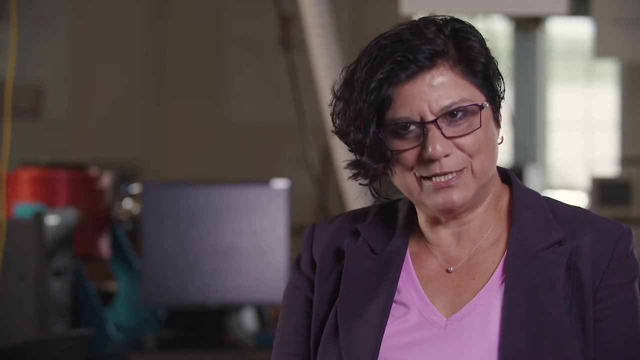 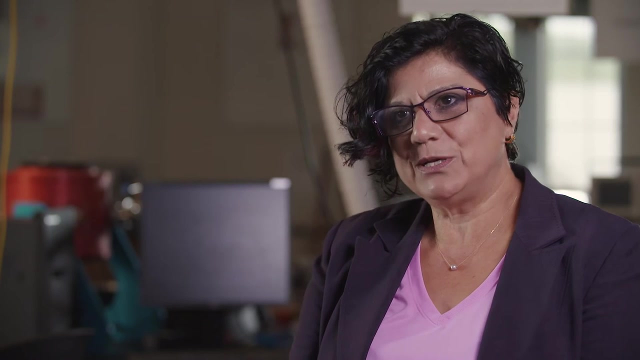 study is just making contributions. We are at a point in knowledge that we need all of the other aspects of science to play. So we understand how nuclear reactions take place, what the nuclear physics influences, but we need to know in what kind of environment nuclear physics is operating in, And that's 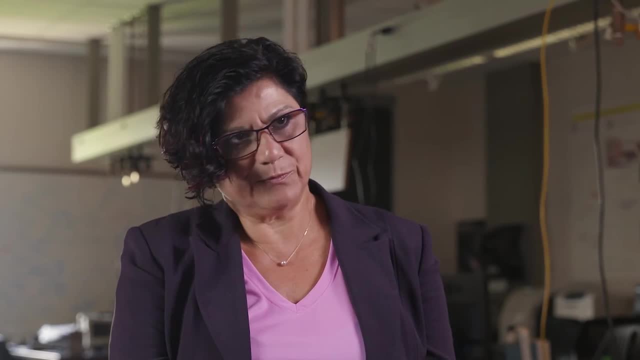 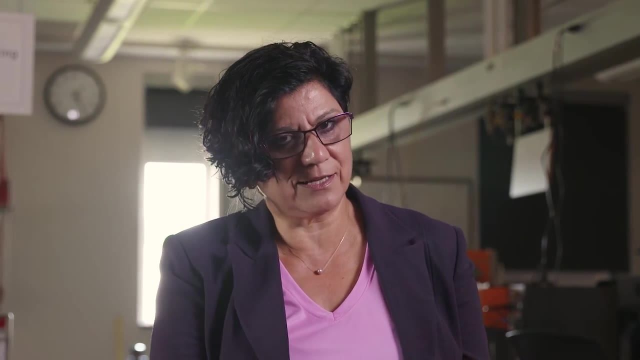 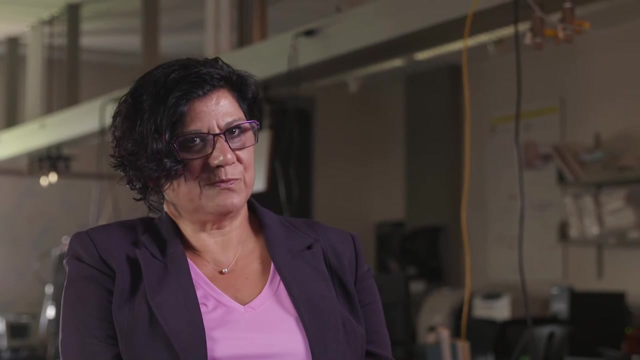 the major focus of my research here. I'm here in collaboration with Rebecca Sermon on the theory side and with the group at Argonne on the experimental side, but also MSU and UBASCULA. Rebecca is a nuclear theorist with special interest in the nuclear astrophysics side. 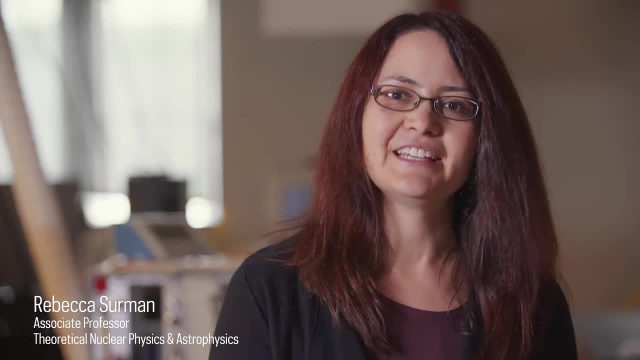 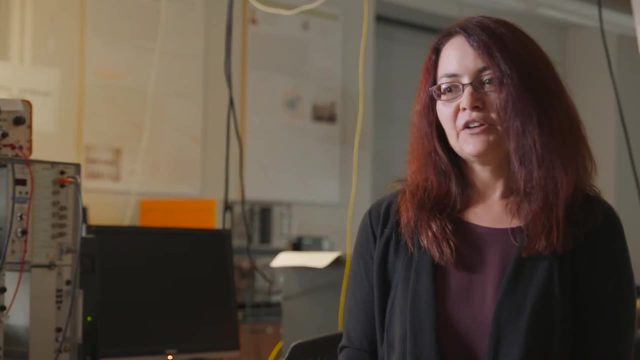 One of the major open problems that I'm working on these days is the origin of the heaviest elements in a process called rapid neutron capture or our process, nucleosynthesis. The question is: where do the neutrons come from for this rapid neutron capture process? 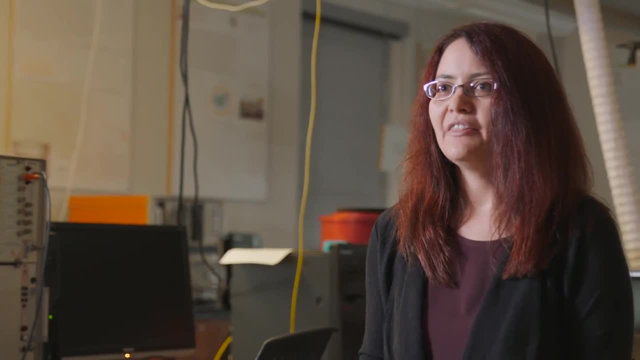 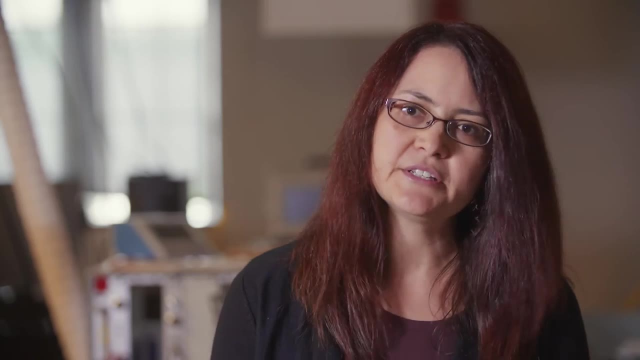 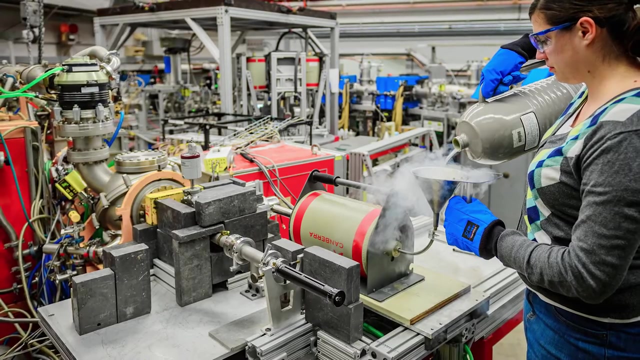 Basically, my research is to look at this problem in a different angle. I'm trying to say: can we use the ratios of the abundances of heavy elements that we see in the galaxy to tell us where the astrophysical site is? Why haven't people done this in the past? Well, the problem is that all of the nuclei created in this event are very far from stability, and most of which have never been seen in the laboratory. Therefore, we don't understand their nuclear properties. We have to model them, and those models have large uncertainties. 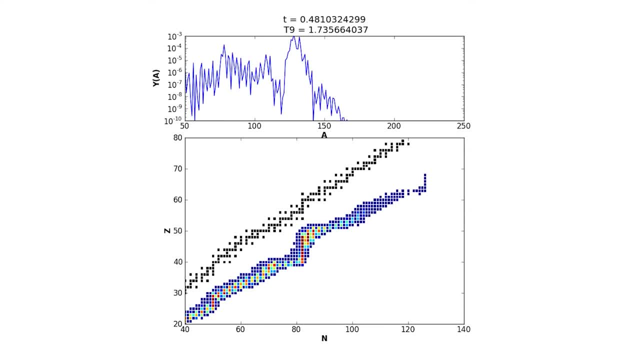 One of the things we've been working on recently is to see what effect do those nuclear uncertainties have on our predictions for these astrophysical environments. We're heading off into two different directions. We want to look at number one. what pieces of nuclear data do we need to? 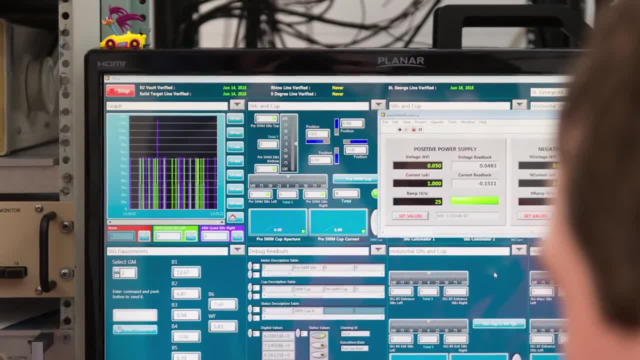 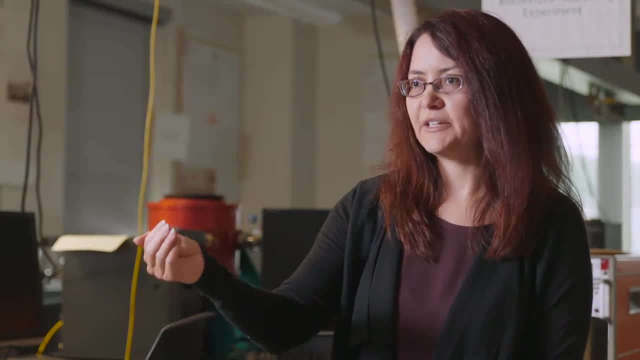 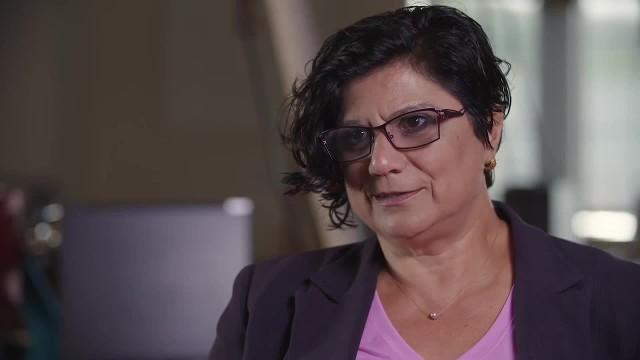 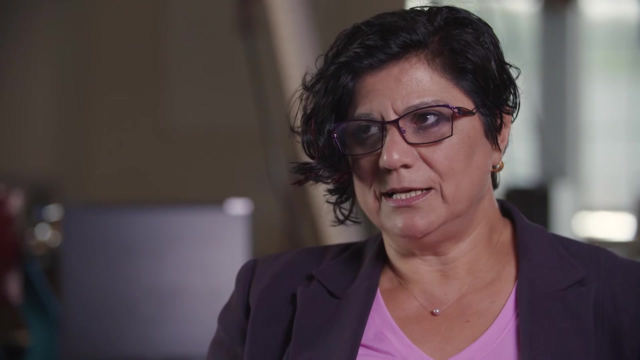 know better in order to make these precision predictions that we need. Assume that we can know the nuclear data better, then how can we use abundance patterns to get at the details of the astrophysical site? No scientific effort today is possible without collaborations both nationally and internationally. 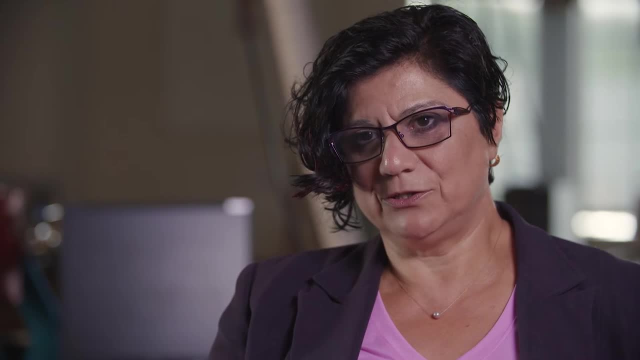 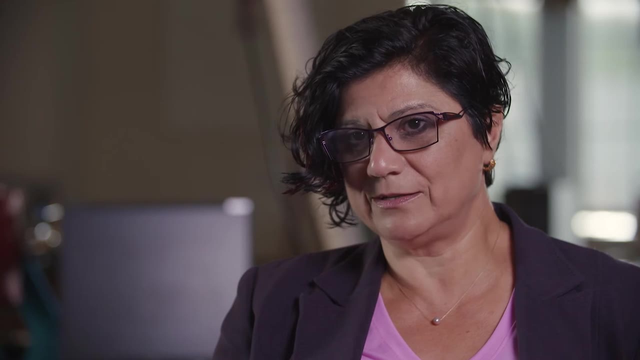 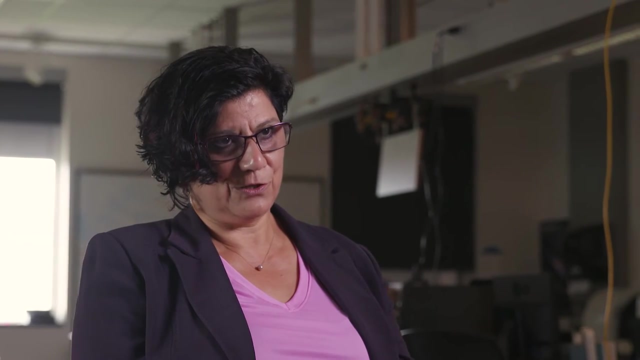 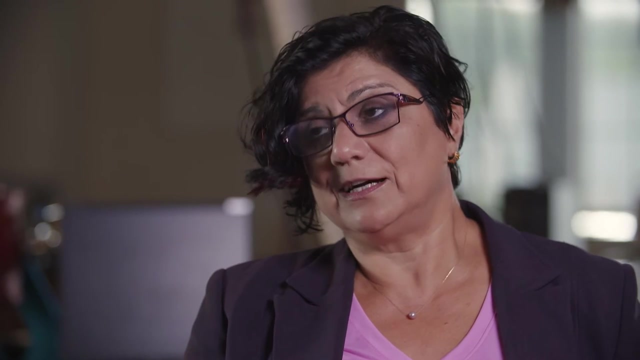 And in fact our faculty at Notre Dame have collaborated with Michigan State in designing a recoil mass separator, SACAR, which is now funded by the DOE. We collaborate in contributing both design equipment and so on, as well as collaborating with otherusing. 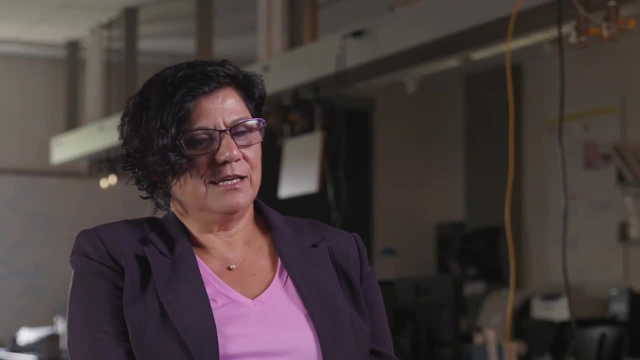 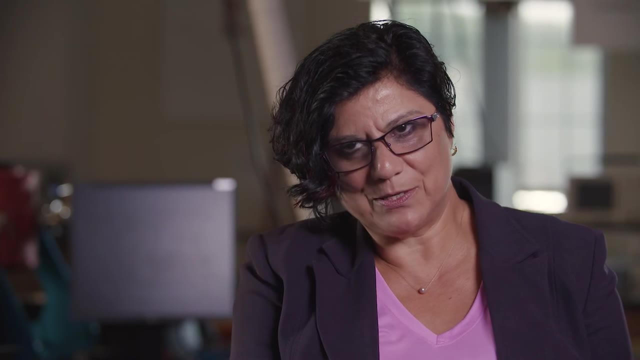 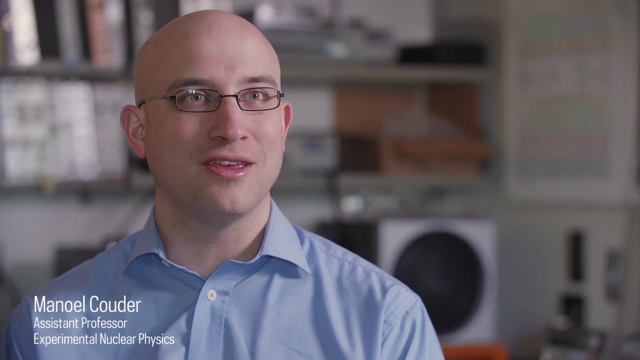 other people's equipment and instrumentation. Manuel Cudert: he is a very key part of installing and implementing the CASPAR program. Right now at Notre Dame, I'm working into two separate projects that are both related to studying nuclear reaction of astrophysical interest in the context of question burning. 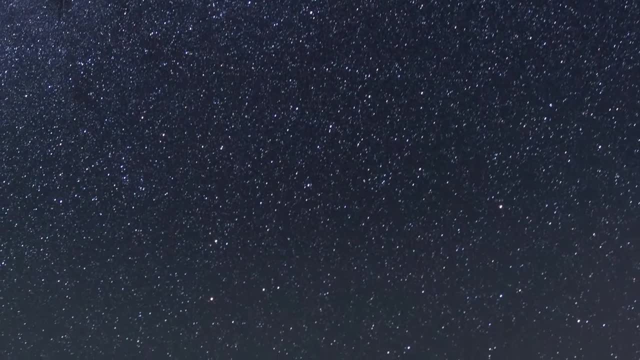 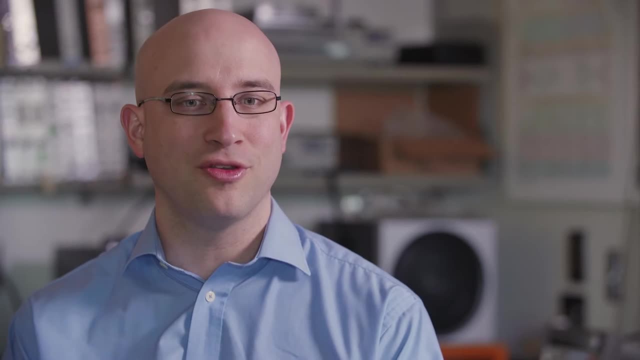 in stars, And so the big questions there are: what are the nuclear reactions that fuel the stars like our sun and bigger than our sun, and what can we learn about the evolution of those stars? And how can we learn about the evolution of those stars and how can we? 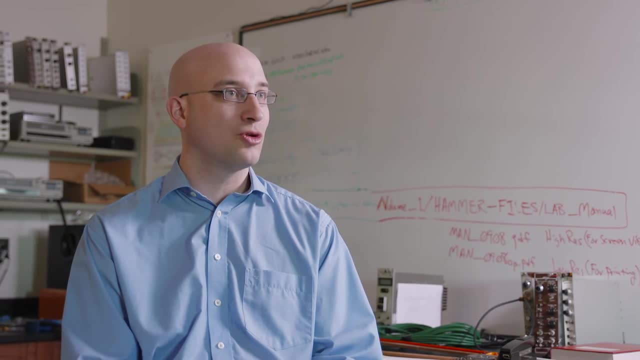 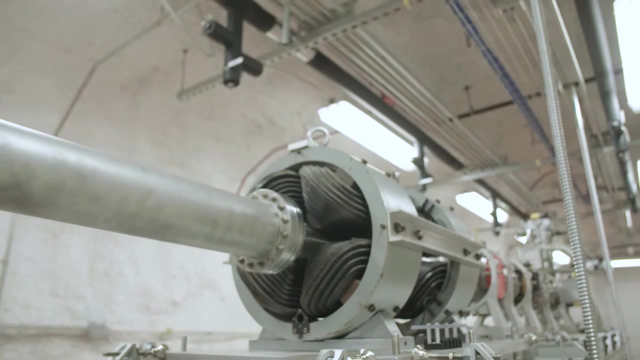 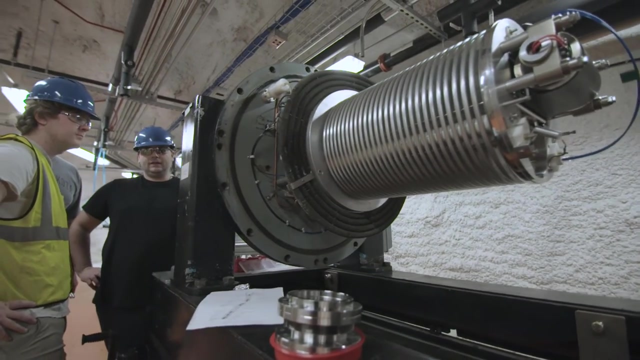 link the observation that our astronomer colleagues make with nuclear reaction that take placethat we believe take place, in those stars. And one way to do that is to continue what our colleague in Italy, for example, did by putting an accelerator on the ground. This is a CASPAR. 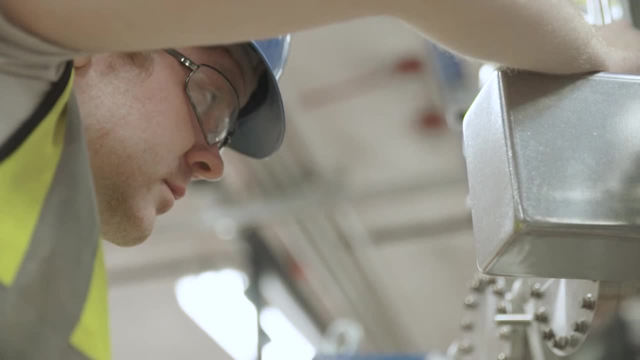 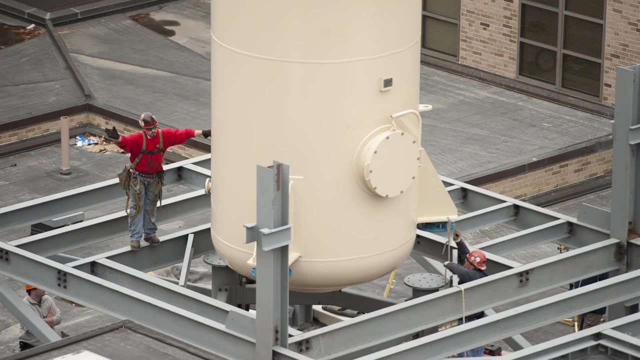 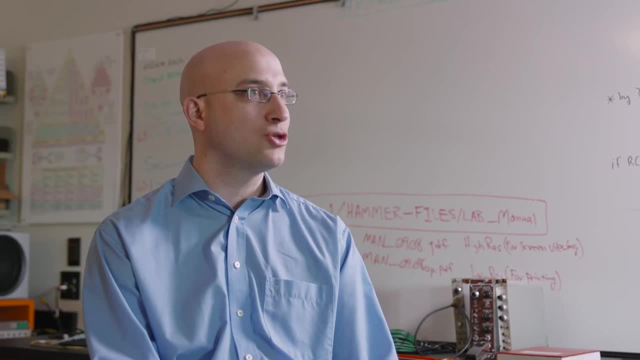 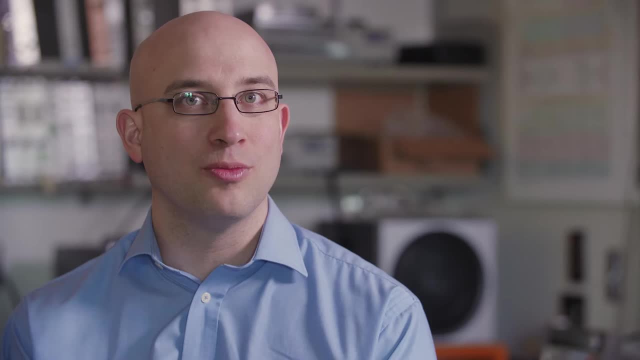 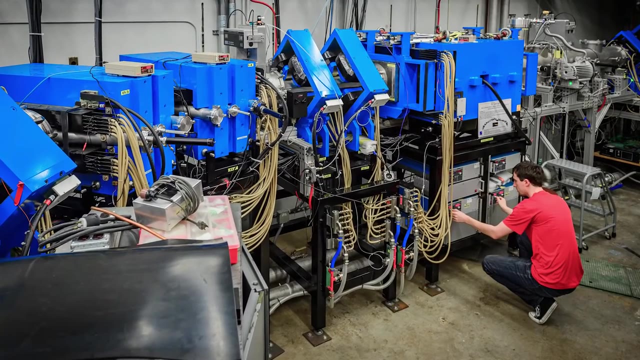 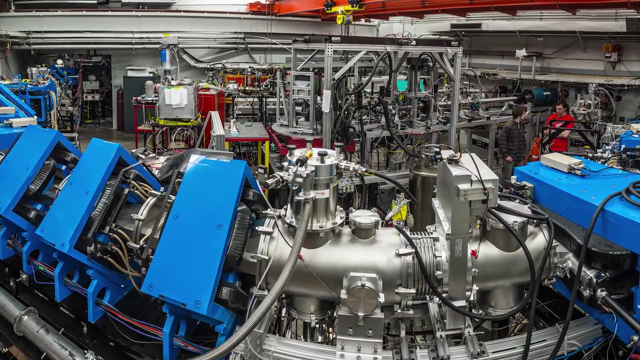 the light target. This allows us to study the production of the charged particle, increasing efficiency, decreasing the background in the gamma spectra. So, in lower mass stars, it is believed that a sequence of reaction coming from carbon leads to the production of the neutrons that are then used to produce theup to 50 percent of the CO2. 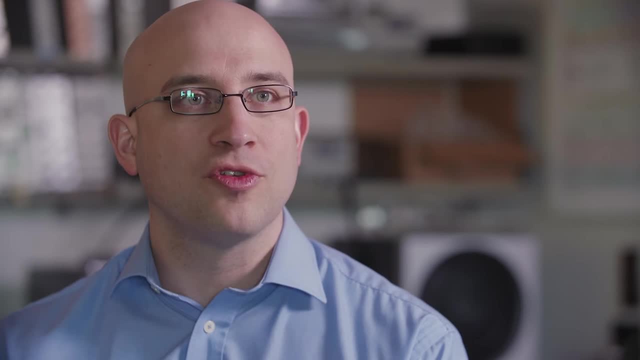 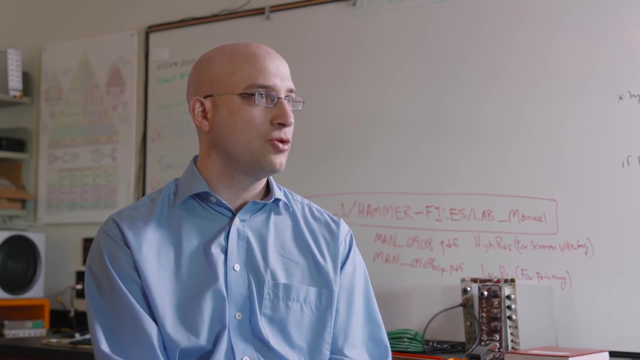 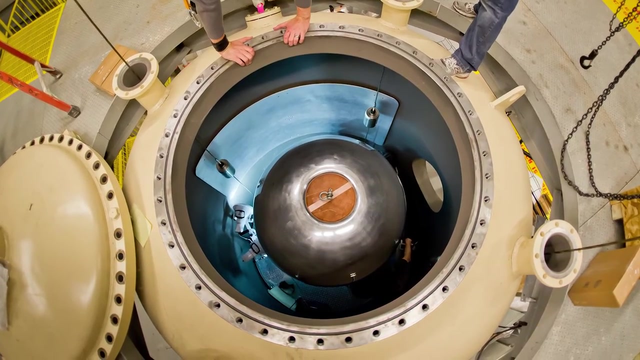 nouvelle base of the element heavier than iron. What St George will do is to study a competing reaction, which is a Neon 22 alpha gamma, and, specifically for Neon 22 alpha, The combination of the high intensity beam coming from the new accelerator. 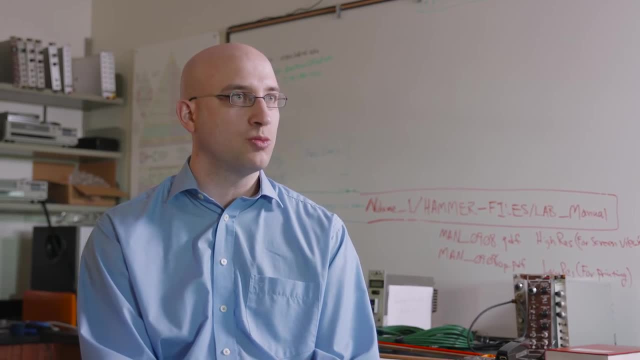 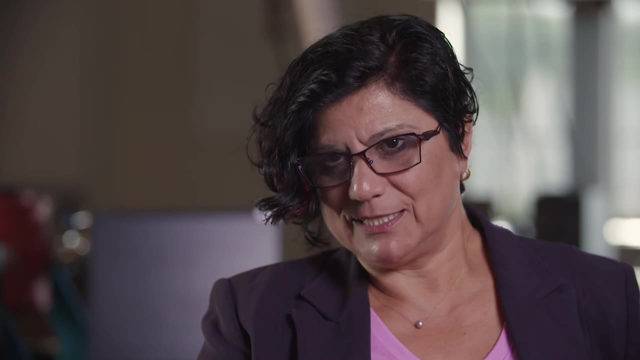 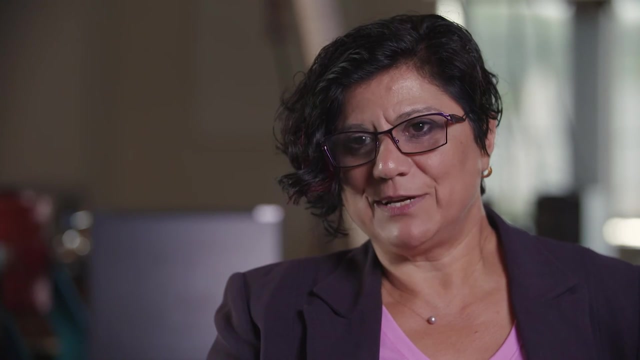 the separation properties of St George should provide us a direct measurement for those critical reactions. Some unique capabilities we have is the radioactive ion beam facility, The twin-sole dual spectrometer. it was the first radioactive ion beam facility in the US. It's a dual superconducting magnet system. 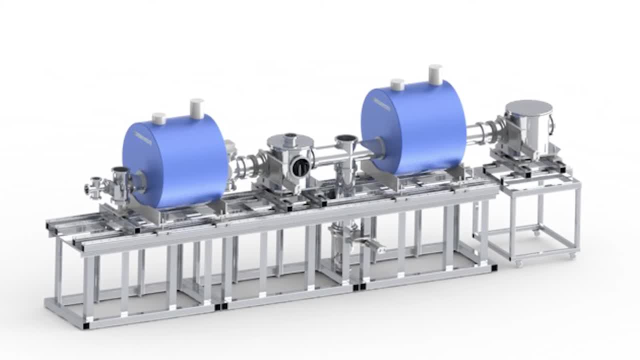 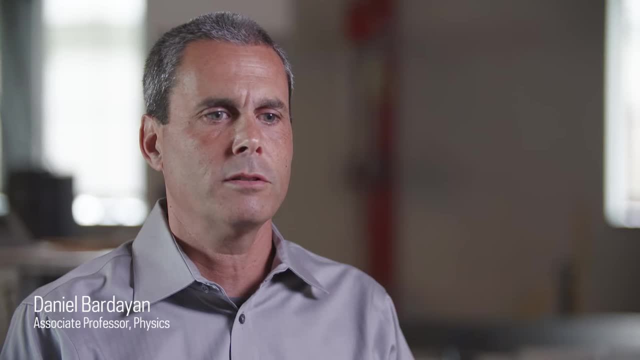 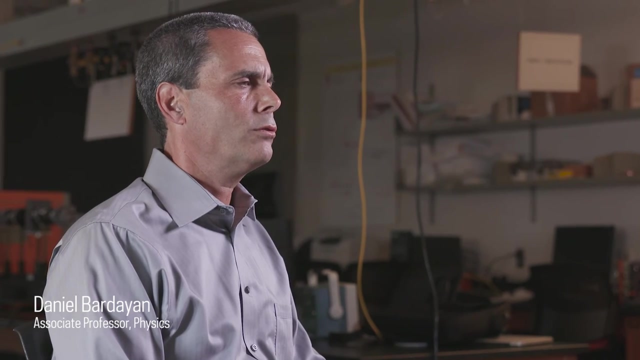 that we can use to do reactions. Dan Bardian is particularly interested in nuclear reactions that involve Fluorine 18 and Neon 22.. The big question I'm trying to answer is why do some stars live seemingly forever, but other stars explore and die catastrophically? 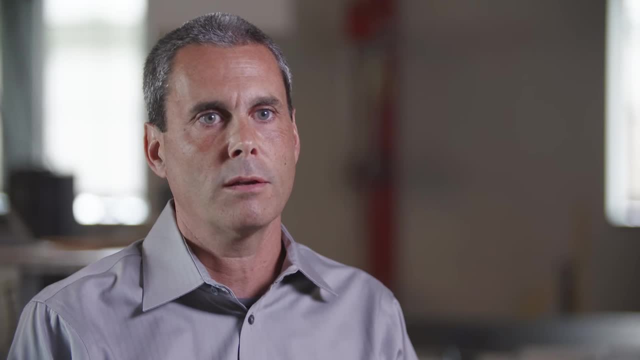 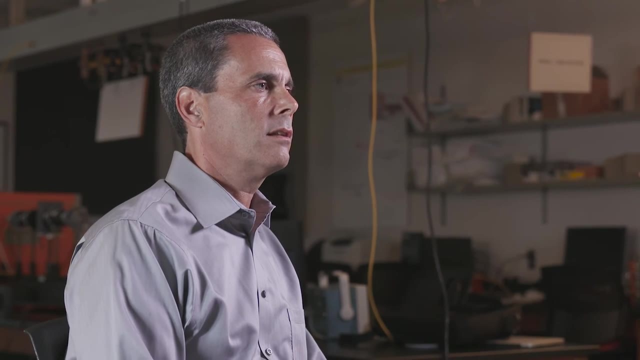 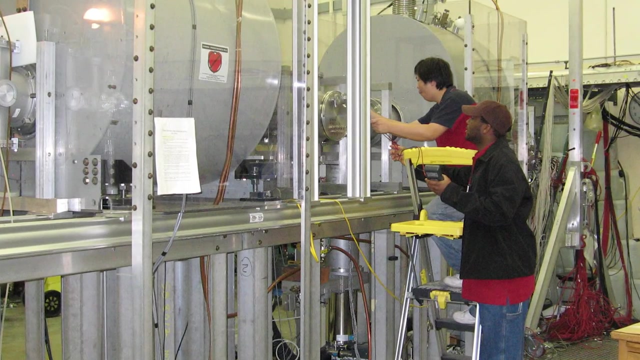 What we study at the Nuclear Science Laboratory here at Notre Dame is the extreme nuclear physics. We produce these exotic nuclei and transport them, separate them with something we call the twin-sole separator. After separating the radioactive nuclei, the exotic ones, we can then measure their reactions. 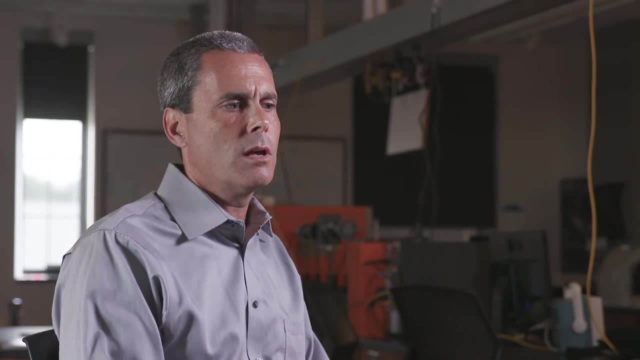 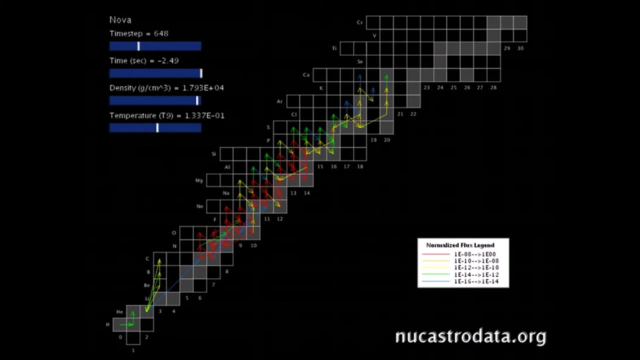 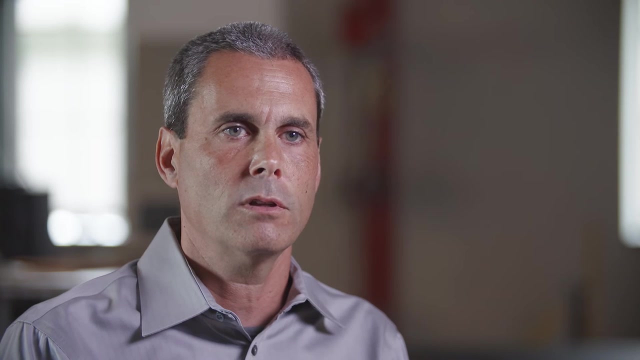 The techniques that we're developing with the twin-sole separator to calibrate proton capture reactions. One of the big questions is: what is the rate of these nuclear reactions? By measuring their properties or by measuring the rates directly using the twin sol separator, we can then 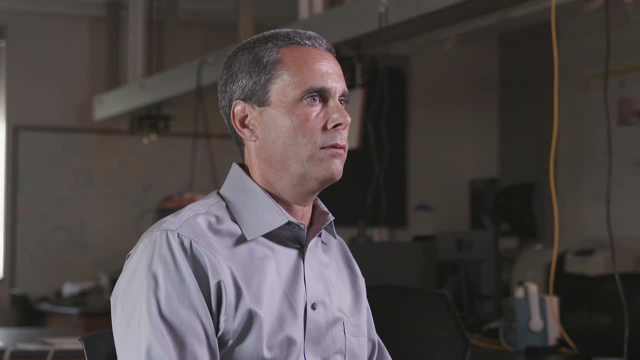 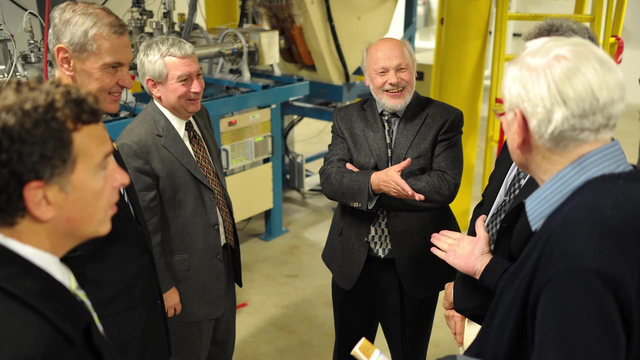 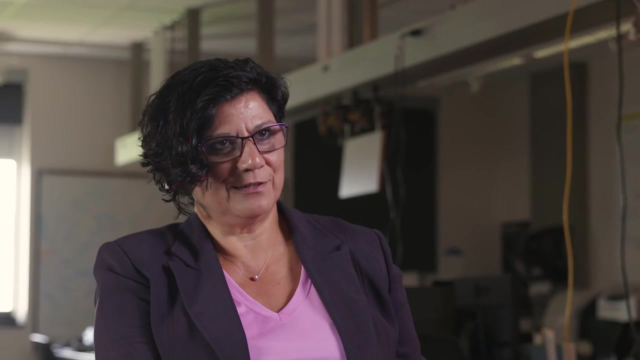 calibrate and determine the astrophysical rates of the very same nuclear reactions occurring in stellar explosions. Notre Dame's support of nuclear physics has been just wonderful. Since 2012, we have doubled the nuclear faculty experimentalists, we've hired a nuclear theorist and, in supporting areas, 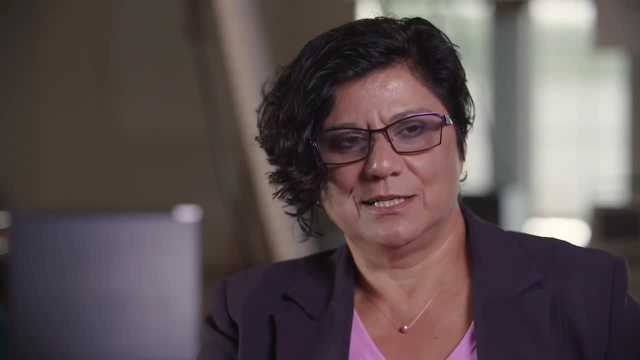 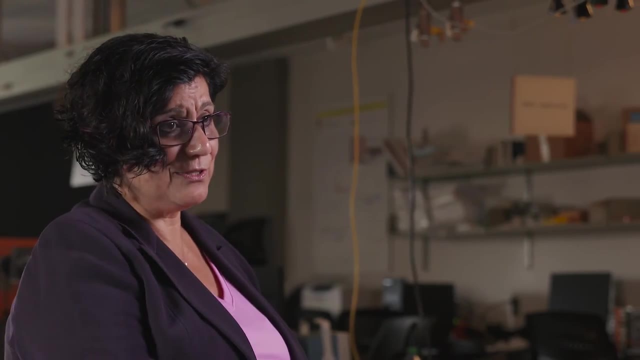 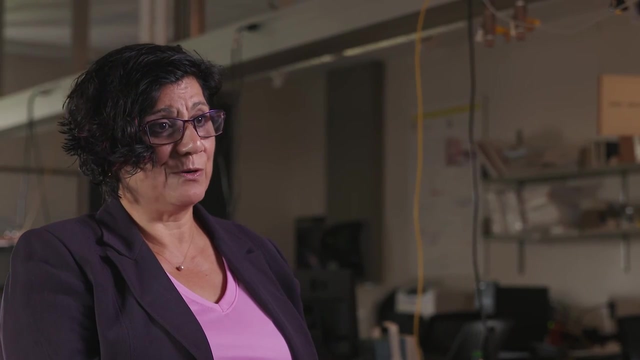 grown in astronomy and so observational area of physics. At the moment we have 35 PhD students in the nuclear physics program, which is a third of the departments and one of the largest nuclear physics programs in the world. We have all of the resources of a major research. 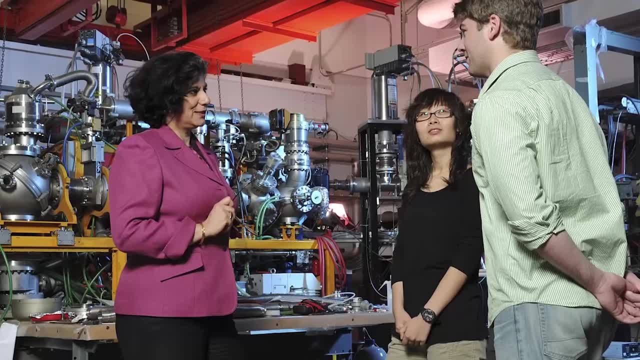 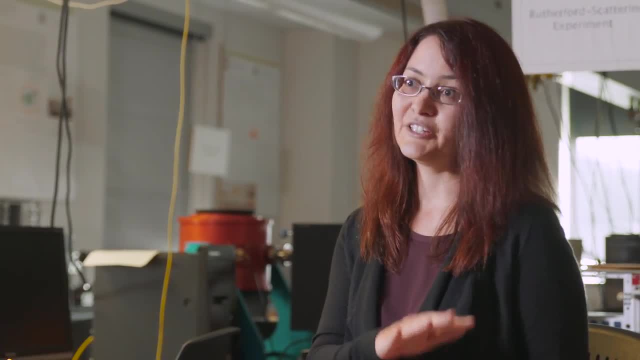 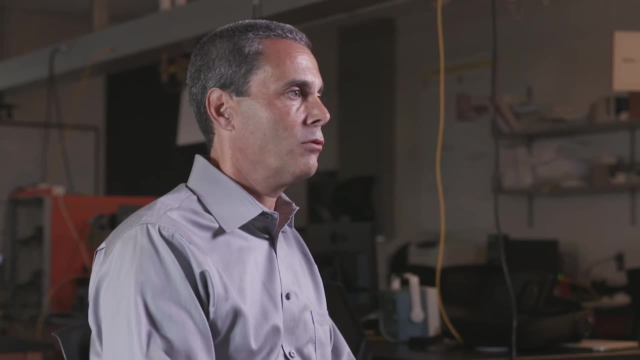 institution, but at the same time, it's small enough to engender collaborations- Collaborations between theorists and experimentalists, between theorists and astronomers. It allows us to quickly try new experiments. I'm guaranteed the ability to try something within two months- sometimes faster- and a lot of 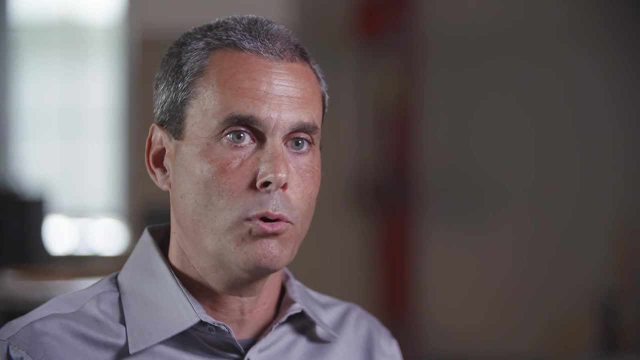 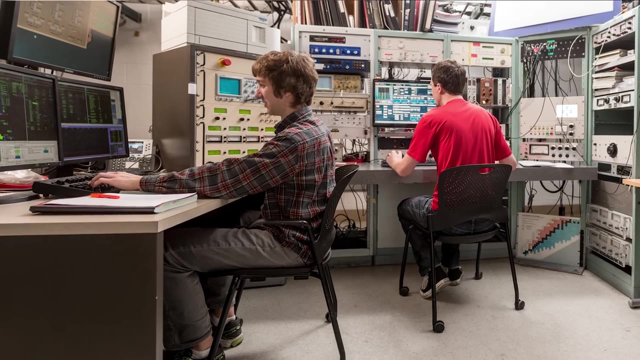 times I can predict the future. I can produce the exotic nuclei that are so important for my research within just a matter of hours. Being at Notre Dame has allowed me personally to grow my research, to grow in the direction that I want to grow, and speed, that's only. 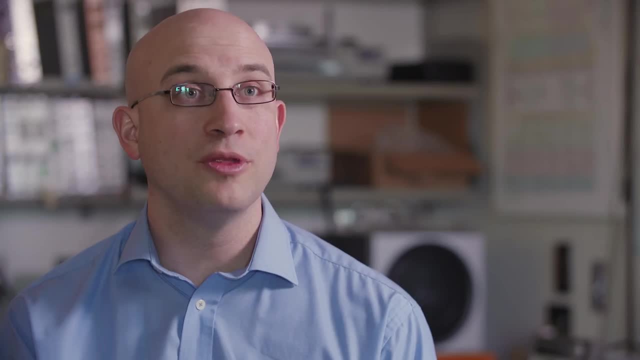 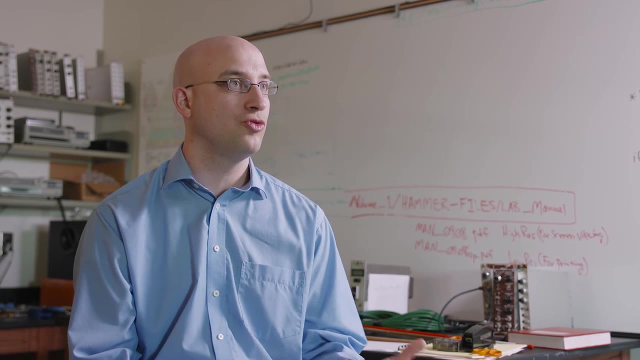 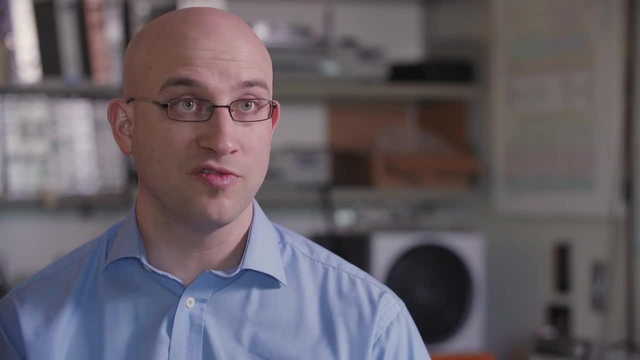 Critical to keep the field going and to produce new science. We talk a lot about chemical science in the term- in term of nuclear. we talk a lot about chemical science in the term- in term of nuclear astrophysics that we do here at Notre Dame. 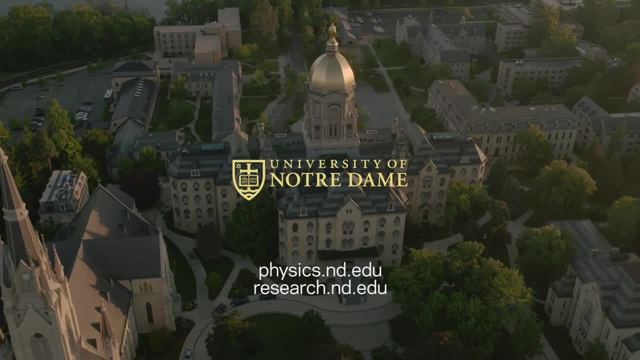 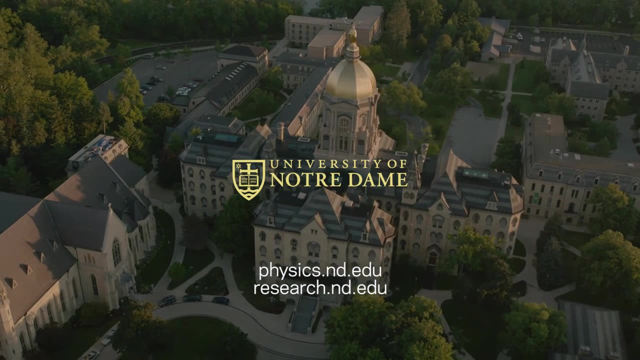 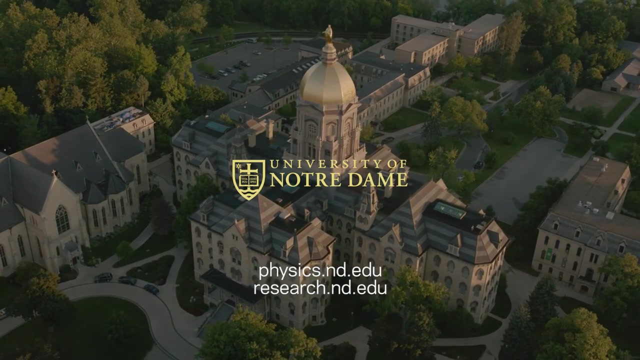 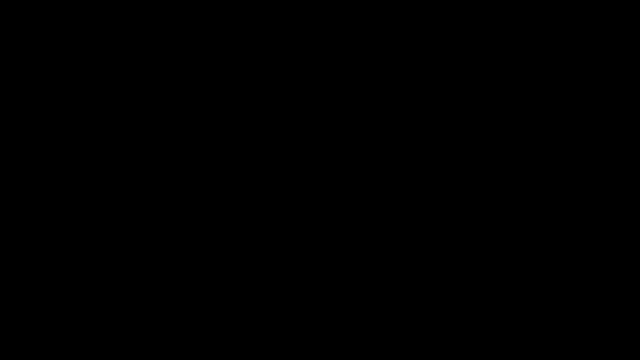 astrophysics that we do here at Notre Dame. www. MontenegrinEUcom. Instagram. Instagram Instagram twins, twins you.